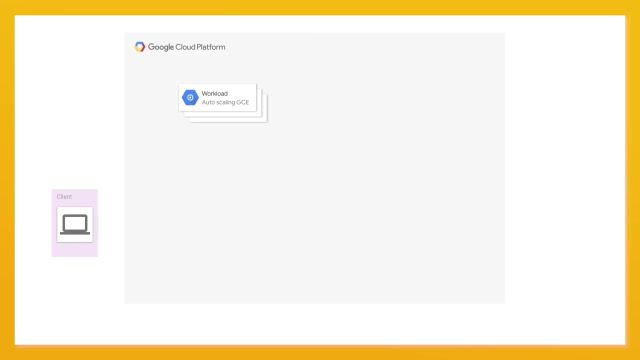 To emphasize these, we used three main techniques: Auto-scaling based on workload lets us make sure that we have the flexibility to scale out heavy workloads on demand, And we use a combination of auto-scale groups Either for preemptable instances and for on-demand. 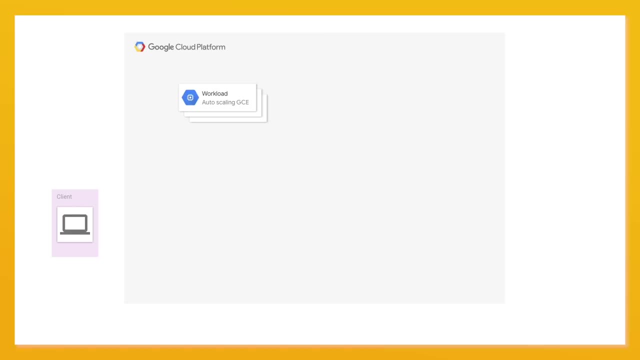 Which leads us to the second point, which is the flexibility to allow us to use preemptable instances as needed, And, thirdly, the option to move stale but useful data into cold storage, again for cost reduction. When it comes to speed, network latency usually has a huge part to play, but Google's network has been pretty snappy in our experience. 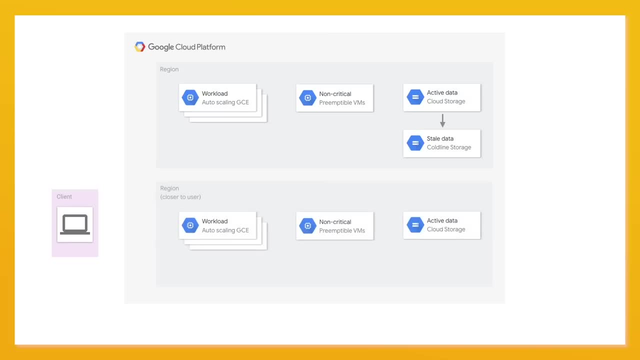 We have been able to keep components that chatter a lot close by within the same region, within the same time frame. We have been able to keep components that chatter a lot close by within the same region, within the same time frame. We have been able to keep components that chatter a lot close by within the same time frame. 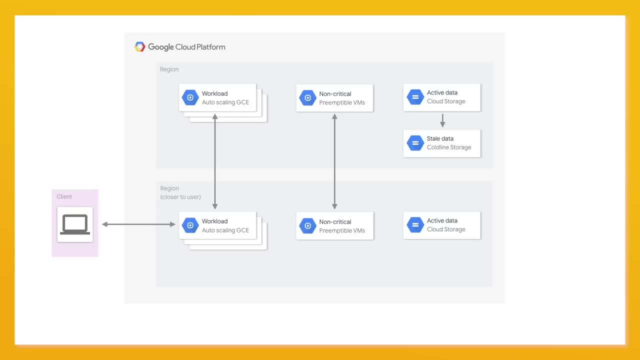 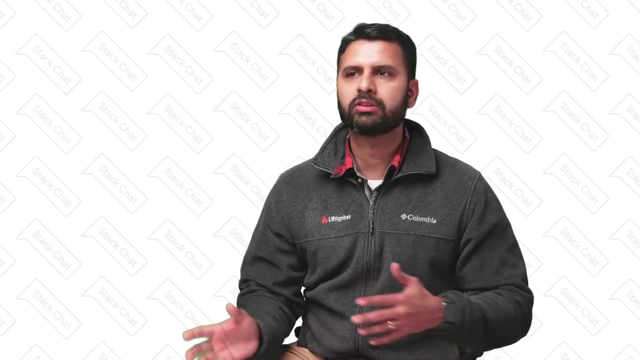 With enough redundancy With Google's footprint, we're able to create and run services closer to the edge, so that all the customer-facing services perform really well, And we've also been able to avoid any outages that will affect our SLA, thanks to Google Cloud. 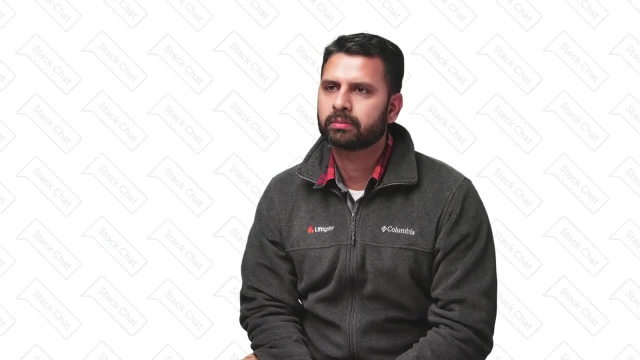 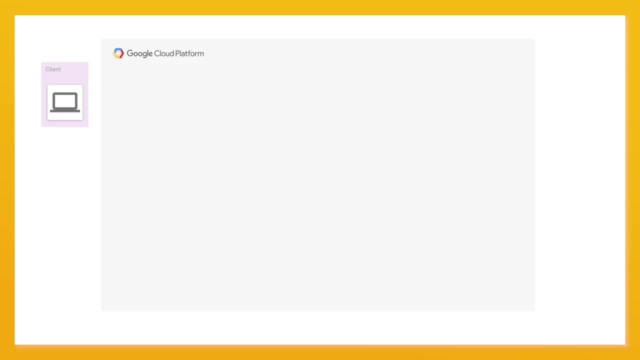 Can you tell us a little bit more about how the recommendation system was actually built? Sure, The diagram is actually a simplified architecture diagram. We are not showing the load balancer and proxies and things like those, but it just focuses on the main components and the services that we have in our architecture. 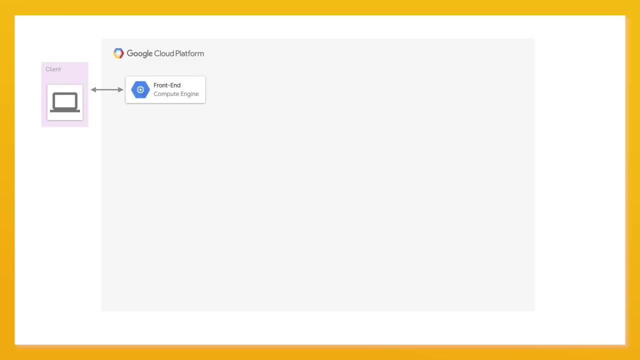 We are not showing the load balancer and proxies and things like those, but it just focuses on the main components and the services that we have in our architecture. The requests to our cloud are either going to hit the front-end APIs or what we call Modelservers. 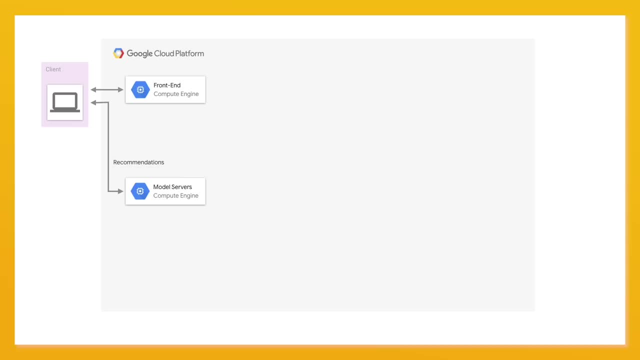 The Modelservers are the ones which, for anything that has to do with user activity and returning recommendations and results, that's taken care of by the Modelservers, where all the magic happens. For everything else, like, for example, updating or creating new inventory items or making other API calls, we'll actually hit our front-end services. 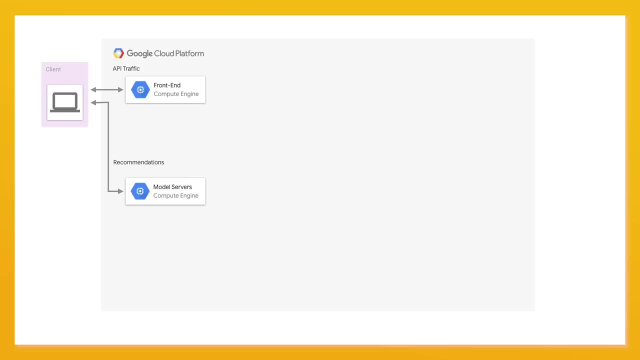 Looking at the front-end services. Looking at the front-end services. When an API call comes in, a bunch of processing happens on those front-end machines and the front-end services. they push the data into data storage. We create either files or other data. push it into some data storage like Google Cloud Storage. 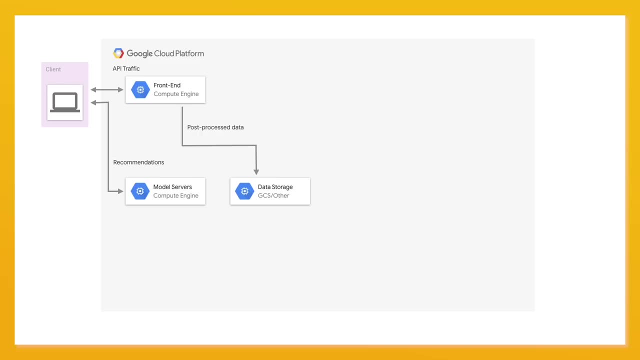 We also have other data stores And GCS would actually trigger an event into Cloud PubSub where we have a lot of subscribers listening on messages on those topics And a subscriber could pick up those, do further processing and an example shown in the diagram is where we have an inventory system. 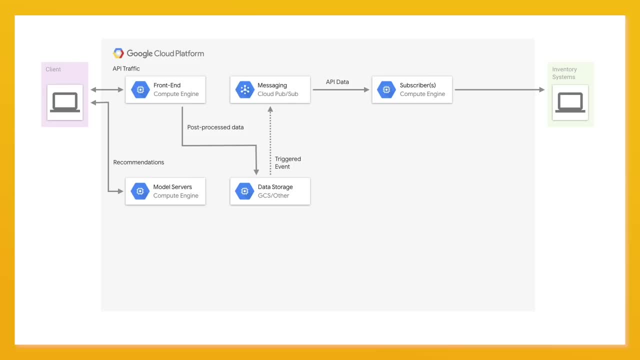 which does further analysis and processing based on what the trigger is. The model servers are the ones, like I said before, which handle all of recommendations and the user activity tracking. They do a lot of processing in-house. A lot of magic happens here. 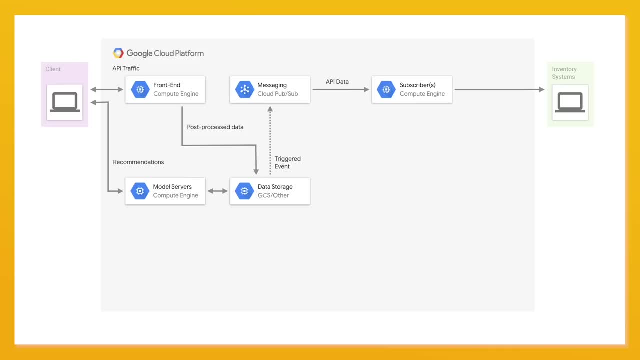 A lot of heavy lifting happens here- Pushes the data once again into data storage. A similar mechanism happens which triggers an event into Cloud PubSub And we have subscribers listening on those topics which pick the data. We have a lot of feedback from GCS. do further processing. 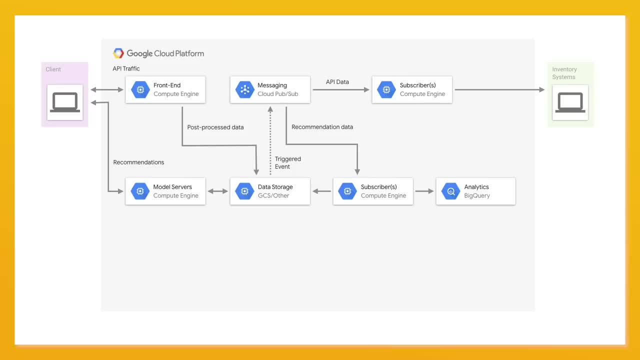 And, as shown in the diagram, this data is now pushed real-time into BigQuery, where our dashboards are fed off of BigQuery for analytics. The key thing here is, while we can move things into BigQuery in real-time, BigQuery can also get a little expensive. 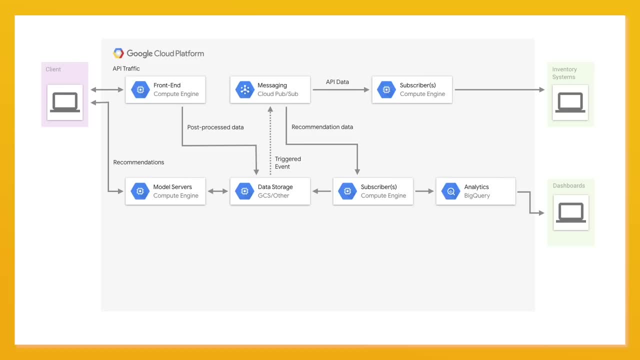 So we want to keep access to BigQuery only when we really need it. So we have an offline processing which takes data off of BigQuery, does further aggregation and then it goes to Cloud SQL which acts like a caching layer. So the dashboards would either hit Cloud SQL or BigQuery. 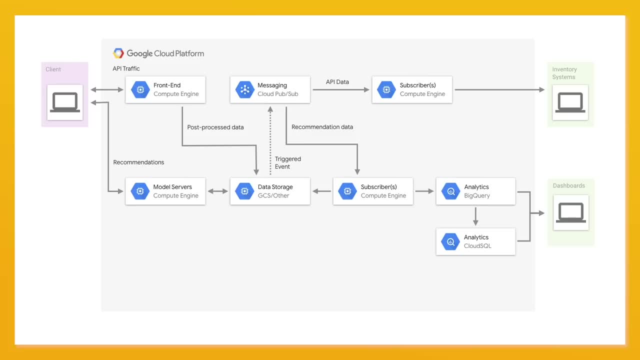 depending on how far back in time they want to go and gather data. The box at the bottom shows our Spark cluster, which runs off of Cloud Dataproc. The Spark cluster is basically used for tuning our models and retraining it for better accuracy. 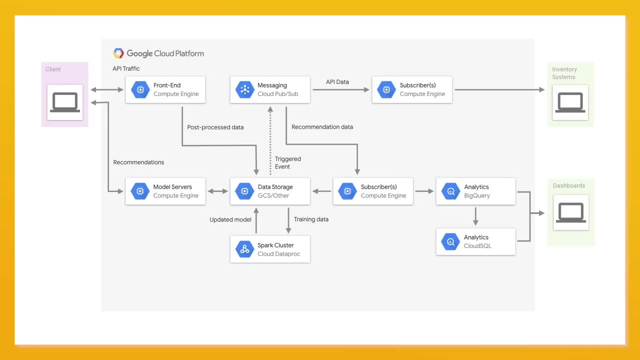 We run it on a nightly basis. We gather all the data from GCS, We have the models running all over again And if the results of those models with the tune parameters are better than the actual data, than what it was before, we make the necessary changes and push those. 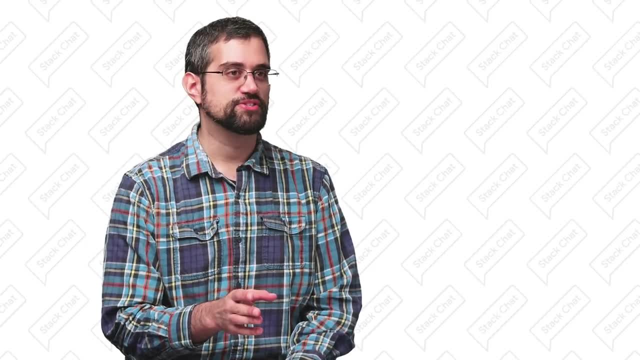 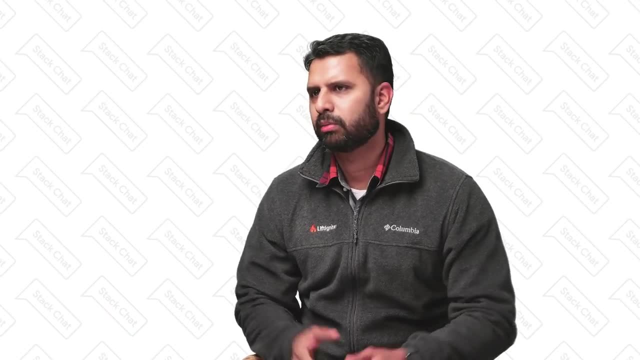 configuration into the club. now it's been a while since you architected this originally. if you could go back and do it again, what would you do differently? we started architecting our platform around 2013, 2014, when machine learning was still not hot, big data was still the thing of the day. it's not. it wasn't as.